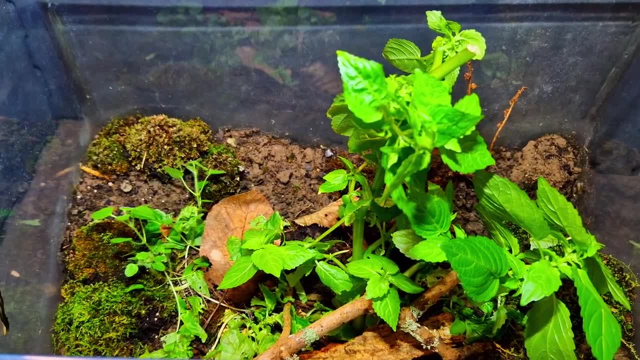 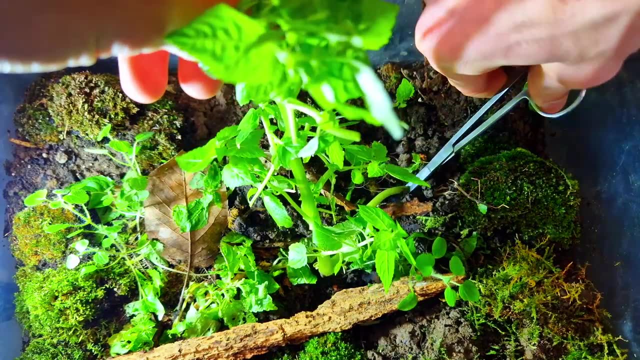 Especially this big plant. It is in the way, so it's got to go Snip, snip And yes, I'm struggling to cut this plant. Don't judge, it's hard and it looks okay. The slugs love to eat this plant. 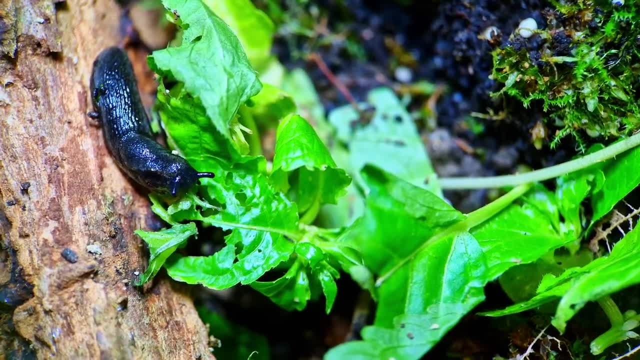 So I'm keeping a part of it to add back later as food. Now I'm going to cut this plant. I'm going to collect some new plants to add in the terrarium, And with plants, of course, I mean moss. 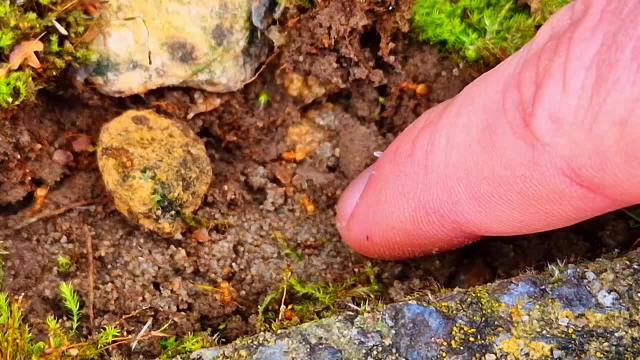 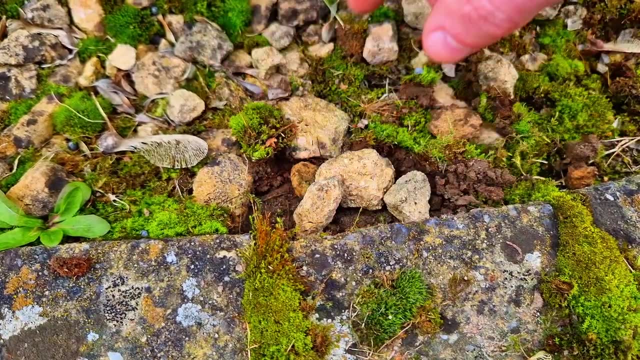 I disturbed an ant nest. Let's see if they are friendly. Ow, Okay, apparently not Covering their nest up a bit, I'll come kill them later. Just kidding, No, I'm not. The substrate in the terrarium has become too compacted. 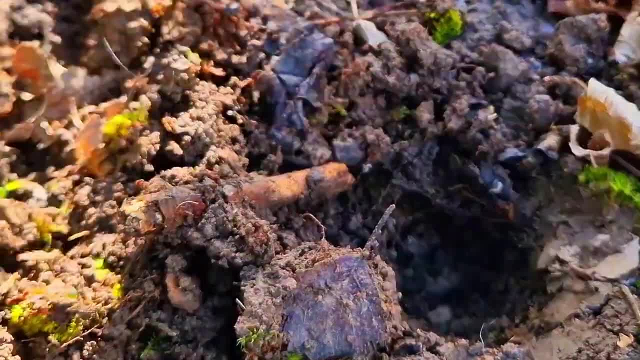 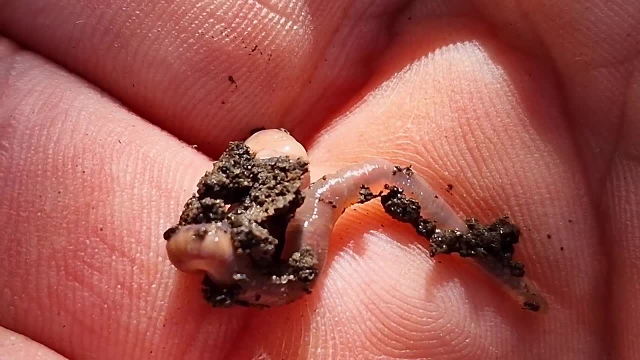 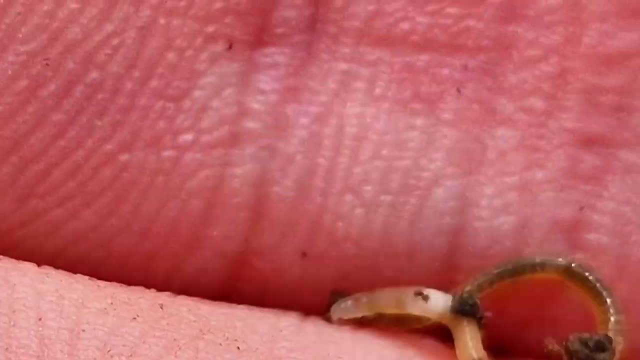 So I'm looking for something that can solve it for me. Earthworms. They will dig through the soil And create more holes. They will also make more nutrients available for the plants. I saw a tiny one. This is probably the size you are more used to. 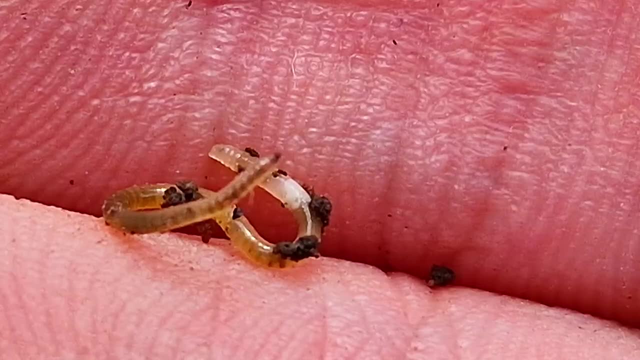 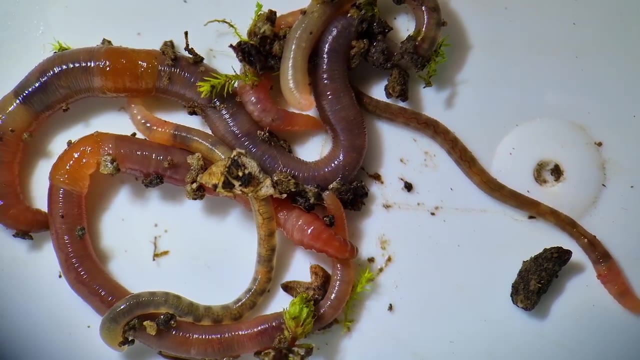 Because it's about the size of your d- I'm sorry. And here it is the sausage party. I will add these in the terrarium later. First, I need to clean up the terrarium a bit more, Taking out all the dead plants and moss. 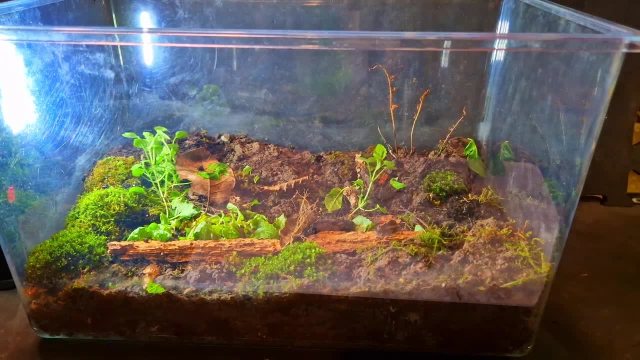 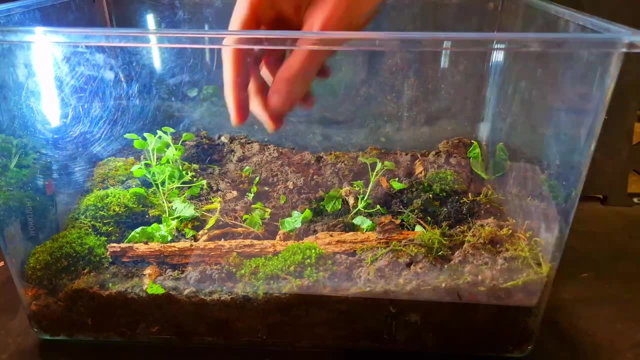 This is not a fast forward, by the way. I'm just that fast, Just like the flagship, Just like the flash. At least that's what my girlfriend calls me. Oh wait, Some animals tried to escape with the stuff I took out. 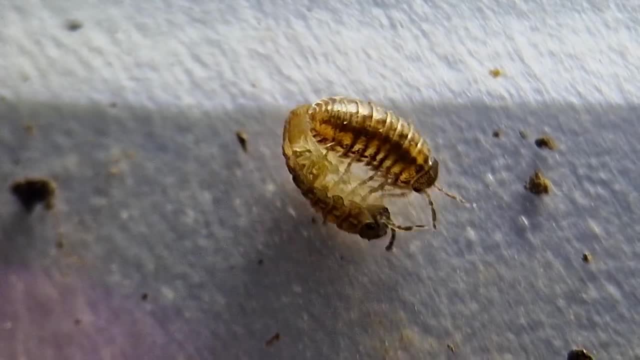 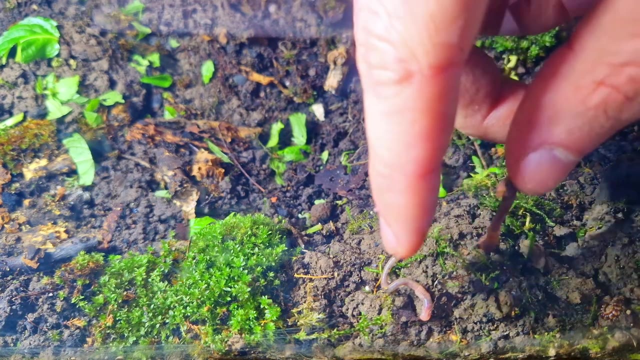 Like these baby isopods. No clue what they are doing, But I will add them back later. First, it's time to put in the worms. Earthworms don't like light, So they will dig underground fast. A lot is going on in this shot. 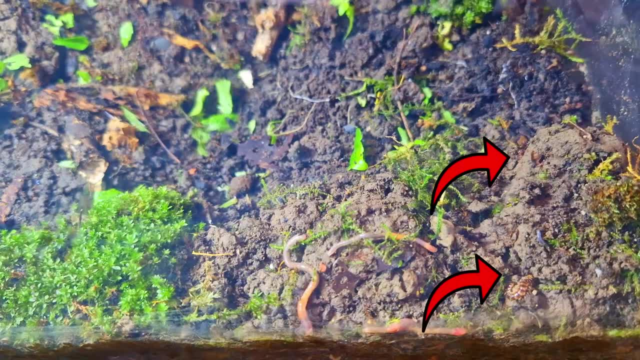 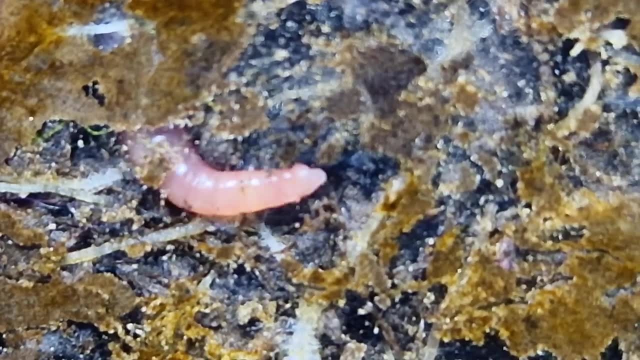 That is a baby slug And those are mating millipedes. Come on, guys, it's getting out of hand. Here is one of the earthworms digging himself here underground. I feel like there is a- that's what she said- joke in here somewhere. 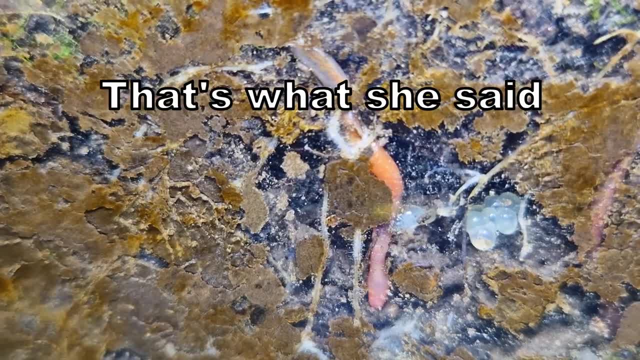 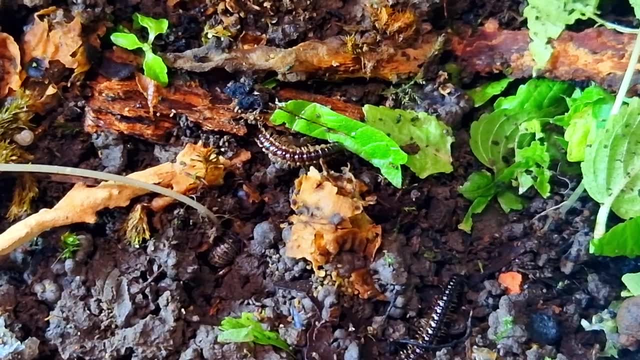 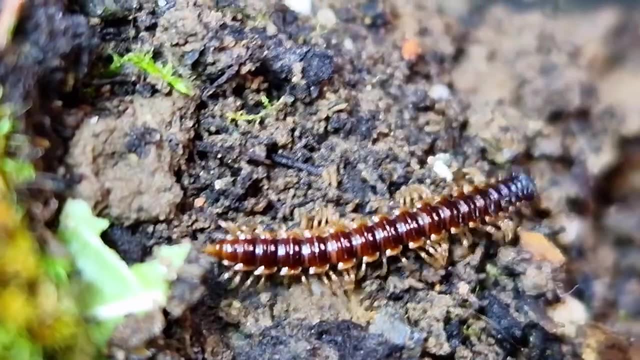 But it's probably going to be too dirty. Now the terrarium is cleaned up a bit, We can spot more animals. I had to look long and hard for a millipede. that wasn't well long and hard. Finally one that isn't mating. 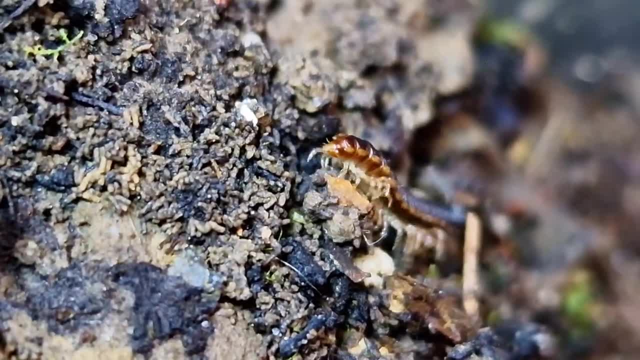 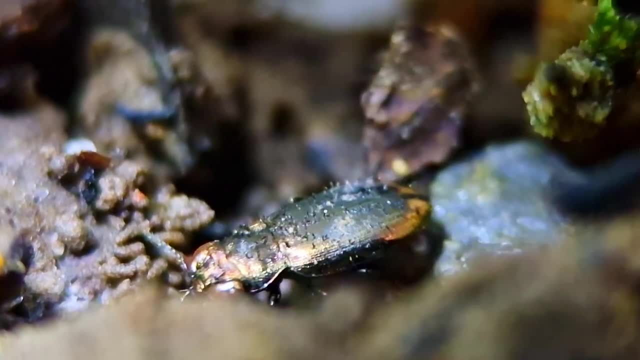 But knowing these millipedes, it is probably looking for a partner. Maybe it can ask one of these two pairs if it can join. This is Bob, the predator of the terrarium, And he has taken an interest in this millipede. 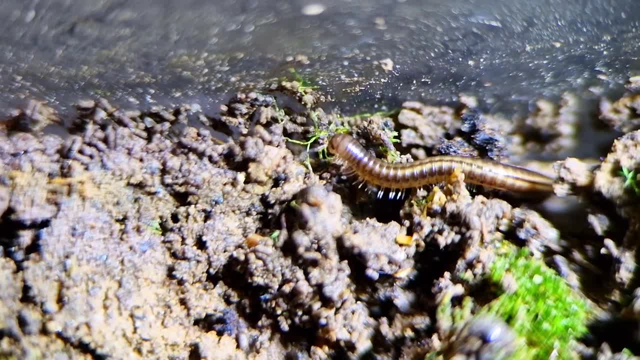 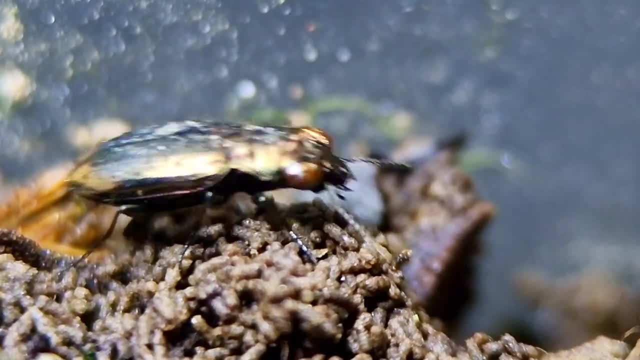 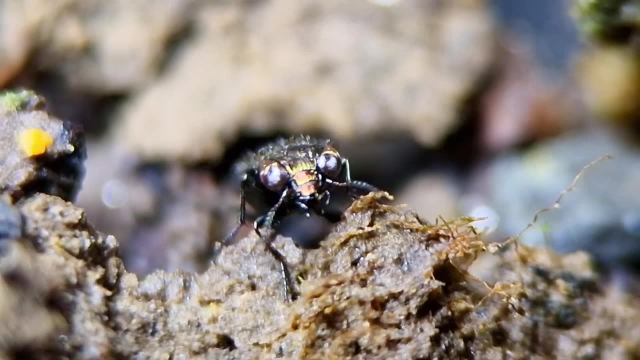 The millipede, however, just want to chill and get out of here. Bob is taking a closer look to see if it's worth it, Apparently not Just chewing on a bit of dirt instead. Yum, Who doesn't want a life like Bob? 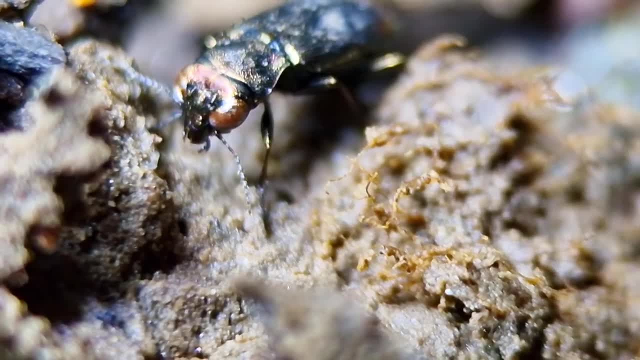 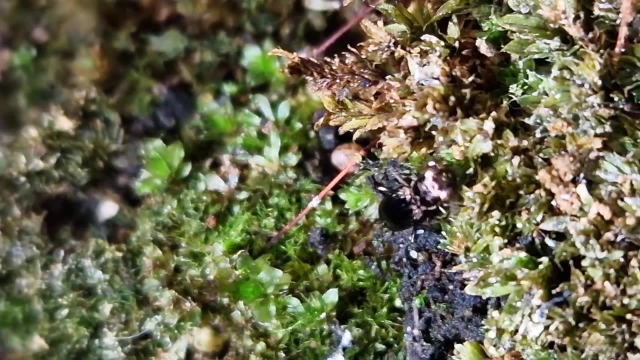 Just chilling Eating. And there is a second Bob in there somewhere. I just don't know if it's male or female. As you can see, Bob is tiny, So it's not easy to film these close-ups. That is why the image is a bit shaky. 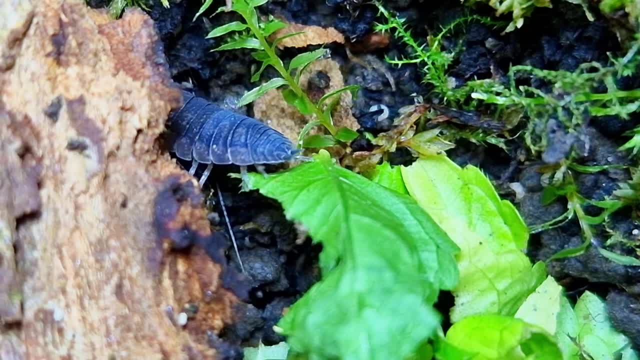 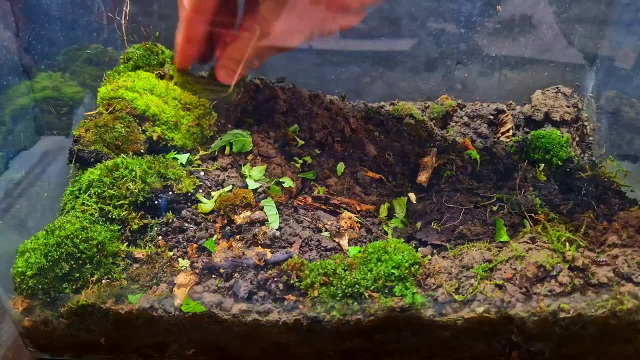 Here is an isopod Later in this video. I still have a trick to lure the animals out, And you will be surprised how many are actually in there. But first let's restore the terrarium. Yup, Here we are again. 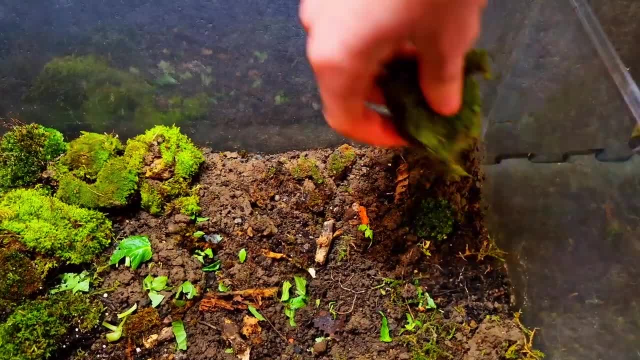 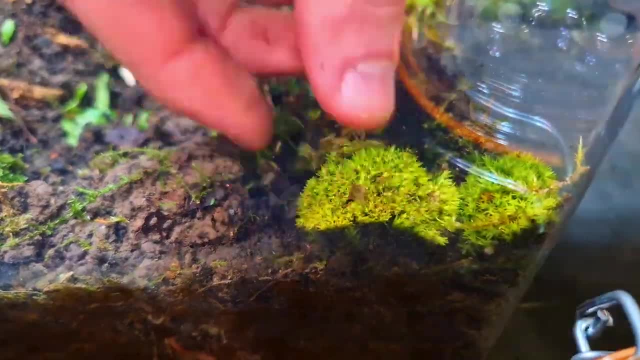 Me adding moss into the terrarium. Don't worry, we'll get through this together. You can do it. Keep watching. I also wanted to let you guys know I ordered a new mic, So next video you can hear my expressive voice better. 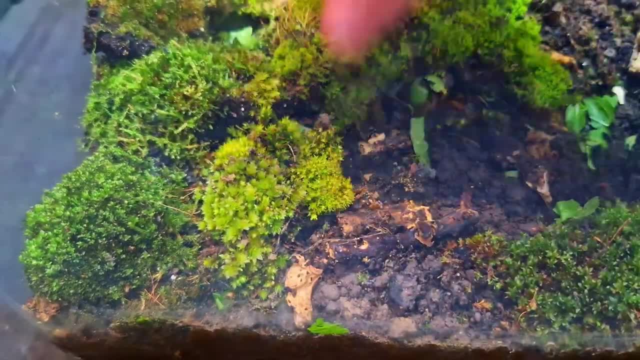 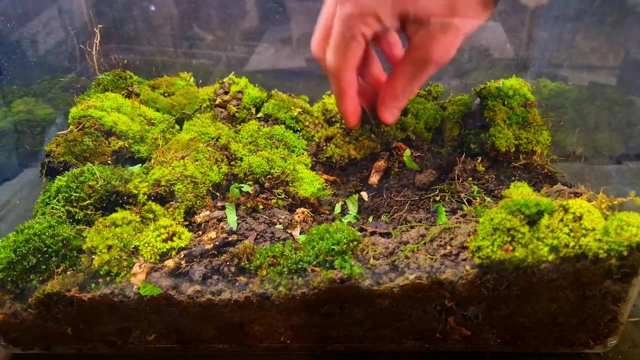 I know you don't want to miss any second of me adding moss, But if you are still here, please consider scrolling down and pressing the like button. Thank you, Almost done. I'm adding some dead leaves and pieces of the plant we cut up before. 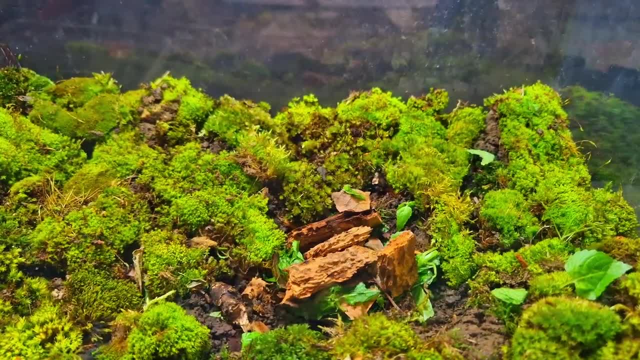 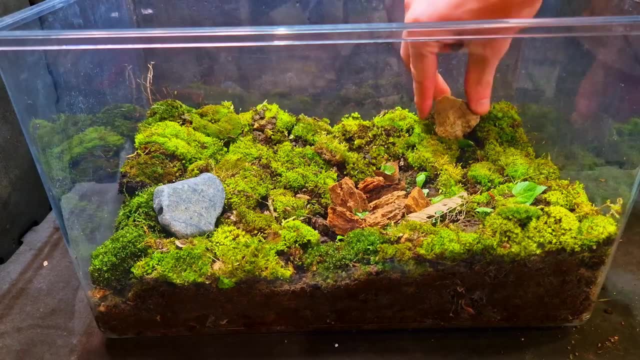 This is great food for the animals. Same with these pieces of wood, The terrarium still looks a bit empty, So I'm adding these rocks. These are just decorative. Yeah, those really lighten up the place. That is not all, of course.